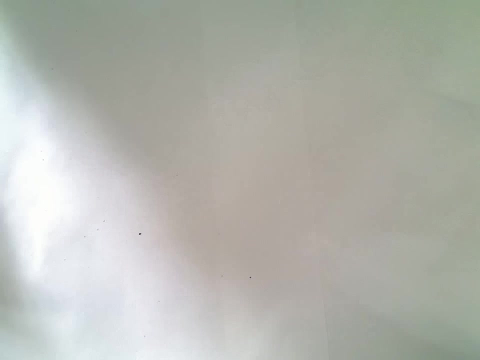 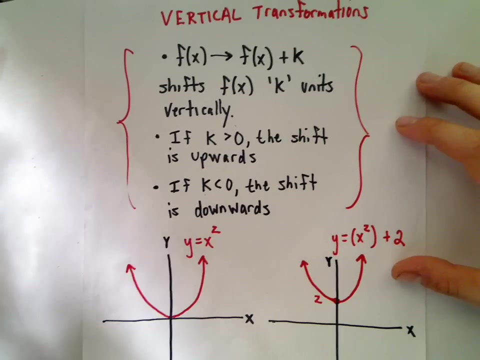 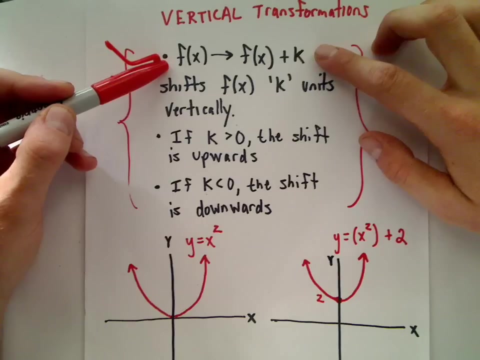 Likewise, we can do vertical transformations and vertical transformations. it's pretty much the same idea. On this one, we're going to basically, just, instead of replacing x with a number, we're just going to add a number onto the outside. So if we add k to the outside, it's going to shift it k units vertically. 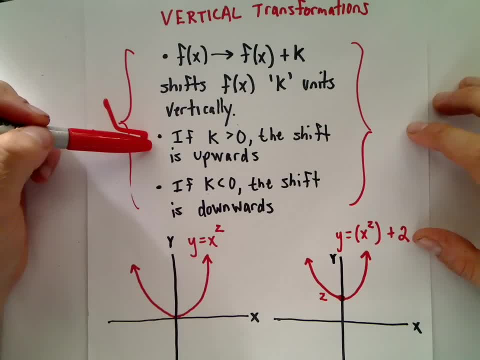 And here maybe it's kind of more straightforward: If the k value's positive, it shifts it upwards, So in the positive direction. If k is negative, it's going to shift it downwards, So in the negative direction. So again here's: y equals x squared. 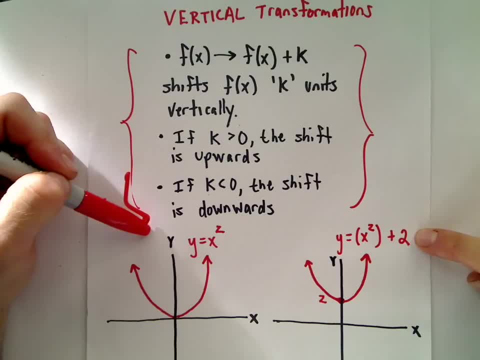 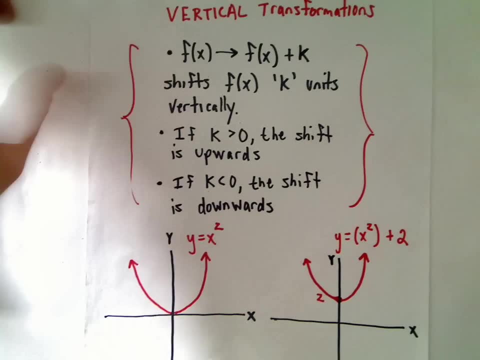 Notice here my original x squared was left alone. I just wrote a plus 2 on the outside. So again that moves that graph up 2 units. So let's graph just a couple here real quick to hopefully make some sense out of this stuff. 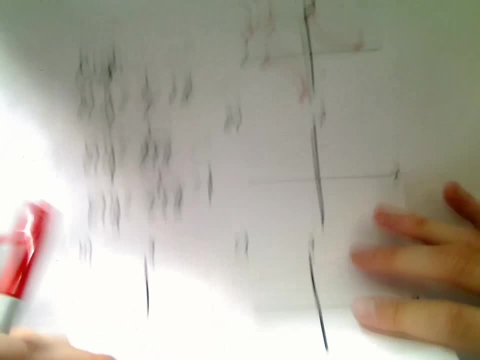 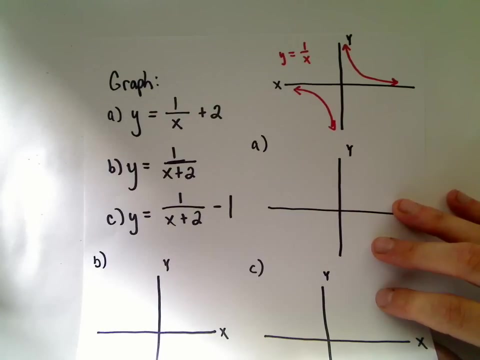 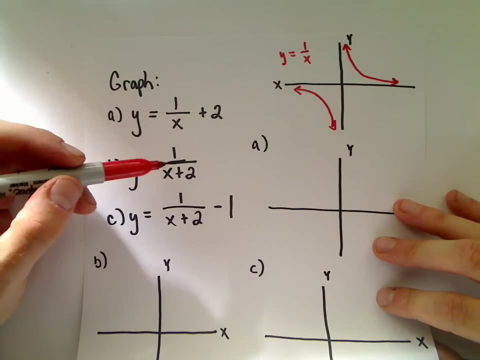 Let me square this, Okay, Let's squeeze it down here a little bit, Okay, So the first graphs I'm going to do: I'm going to graph all a, b and c. I'm going to graph 1 over x plus 2,, 1 over the quantity x plus 2,. 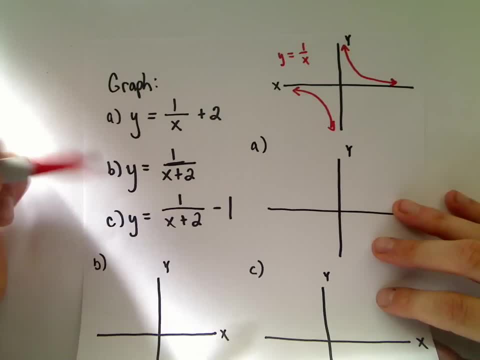 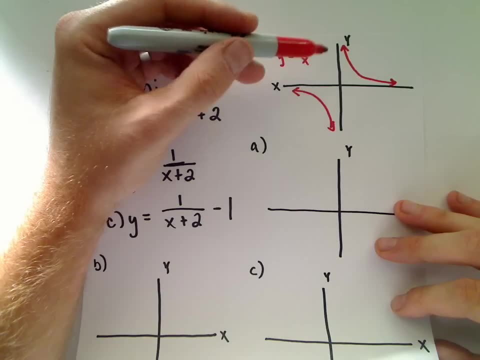 and then 1 over the quantity x plus 2, and then minus 1.. So again. so what we're doing here. we need to know. the basic graph of 1 over x And 1 over x again roughly looks like the one here in the top right. 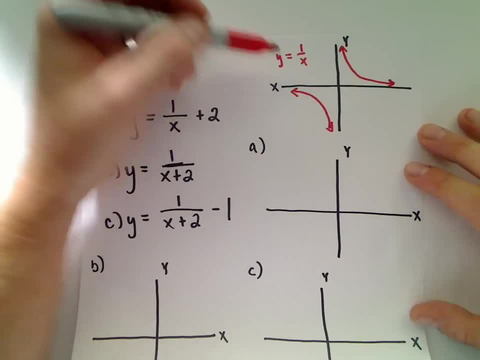 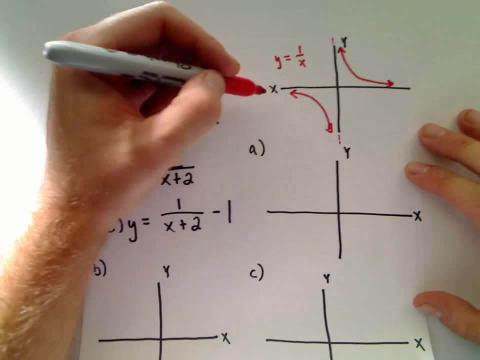 So that's kind of my starting point. I now need to use that to come up with the other ones. And 1 over x has a vertical asymptote on the y-axis And it has a horizontal asymptote along the x-axis. 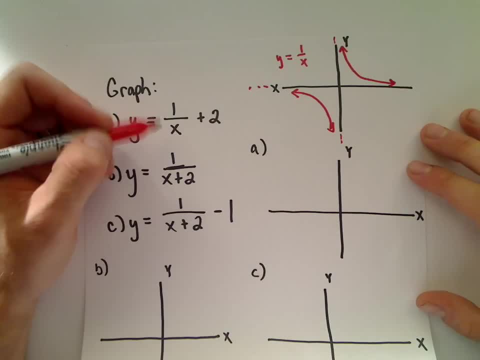 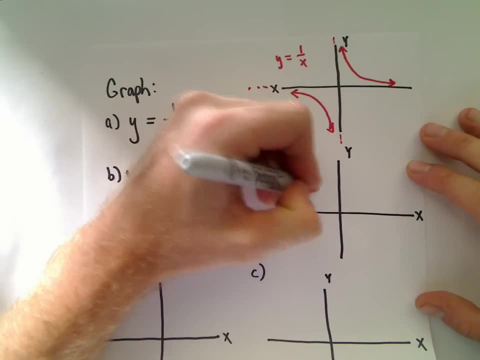 So let's keep that in mind. Well, 1 over x plus 2, all that does is shift the whole graph up 2 units. So my asymptote that was originally at 0 is now going to be at the line y, equals 2.. 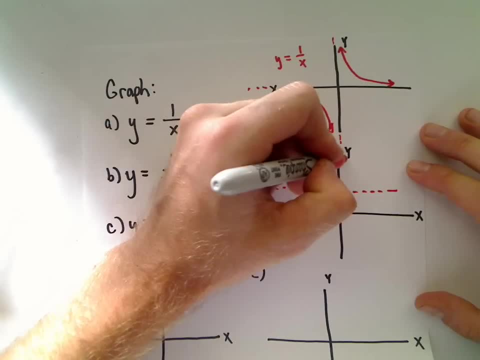 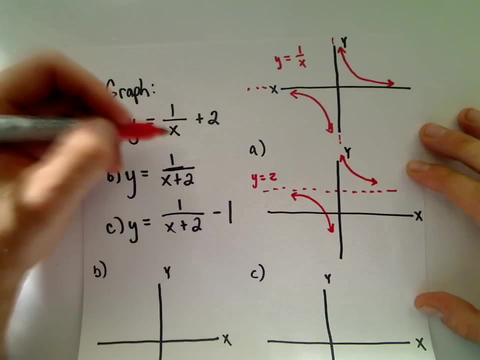 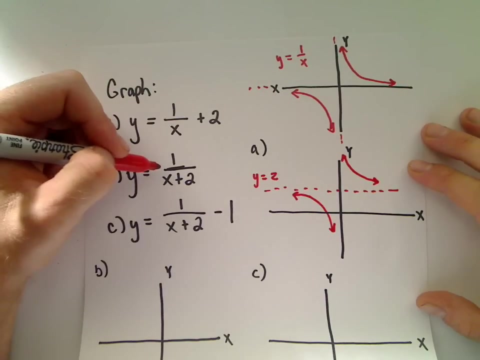 Okay, And again it still has that same basic shape to it otherwise. Okay. So the plus 2 on the outside simply moves the graph up 2 units. Okay, On part b, I have replaced the original x with x plus 2.. 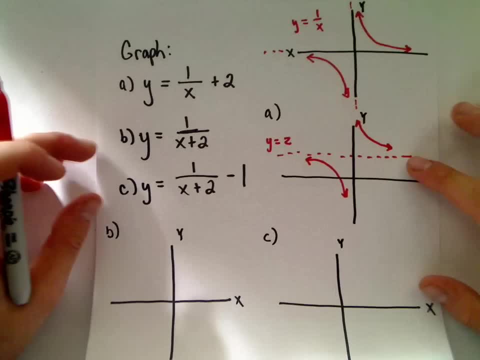 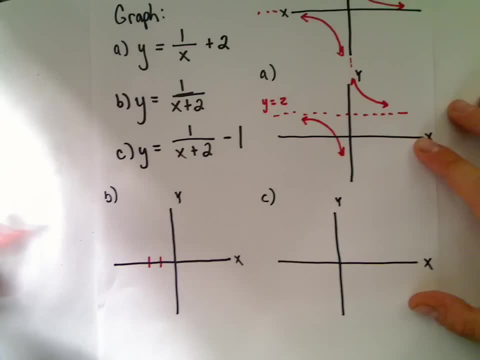 So that's like our very first example. The x plus 2, again is going to shift the graph 2 units to the left. So that means my asymptote that was originally at the x-axis, excuse me, the asymptote, the vertical asymptote, that was the y-axis. 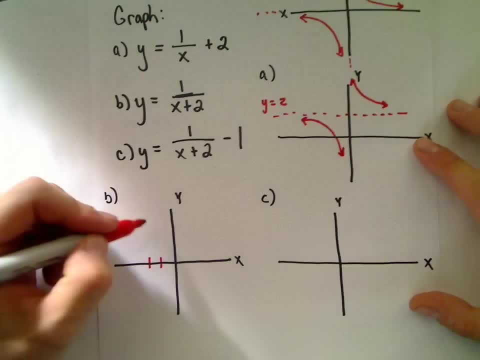 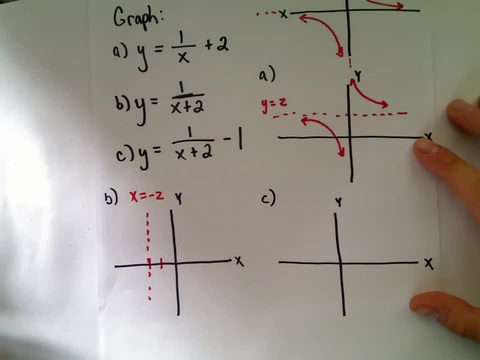 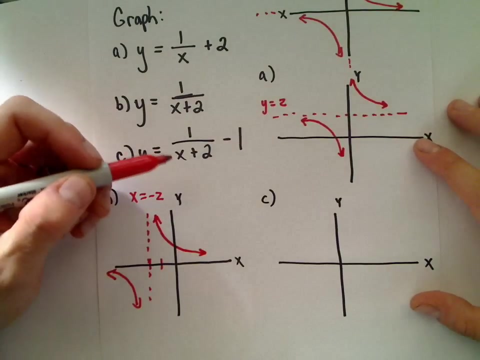 is now going to be at the line x equals negative 2.. And again, otherwise it still has that same basic shape to it. Okay, So again, forgive my rough artistry here. Last but not least, if we want to graph 1 over x plus 2 minus 1,. 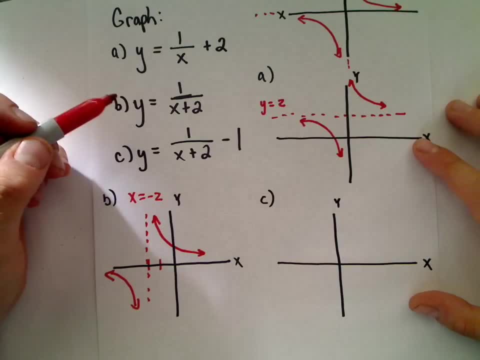 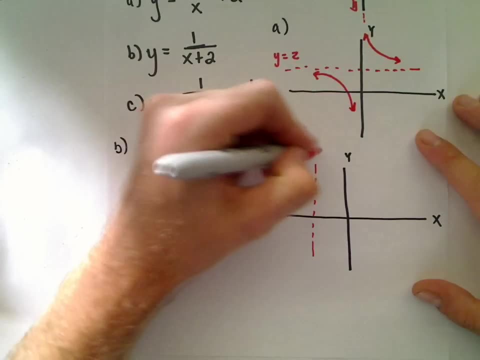 well, all that does is it takes our graph from part b and it shifts it, well, down 1 unit. So we still have the vertical asymptote at negative 2, but now my horizontal asymptote, instead of being at the x-axis. 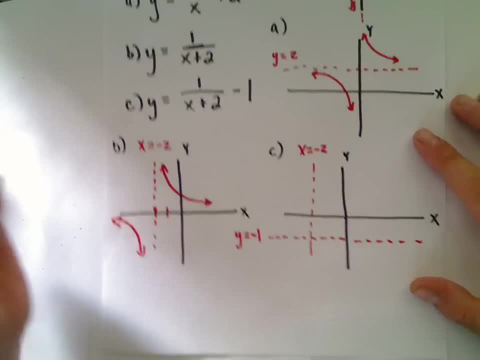 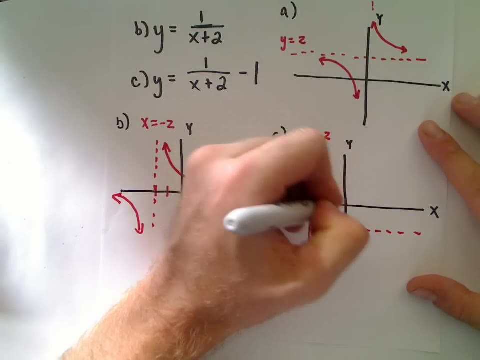 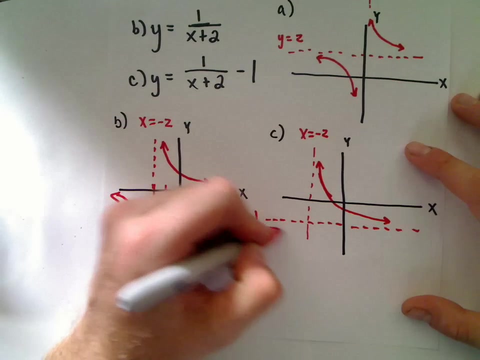 is now going to get moved down to: y equals negative 1. And again, the graph. it should be a little careful. So the graph should cross below what would have a negative y-intercept, But again, otherwise it has that same basic shape to it. 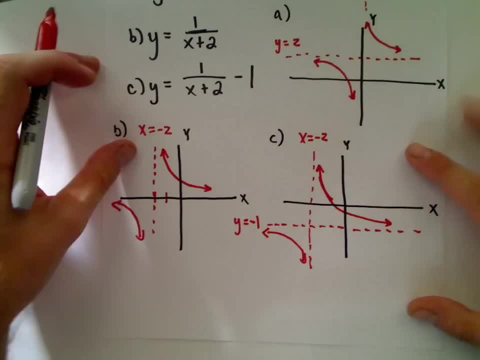 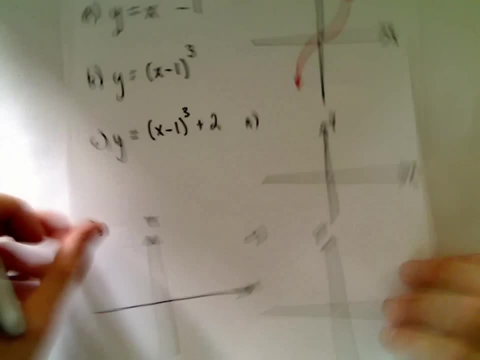 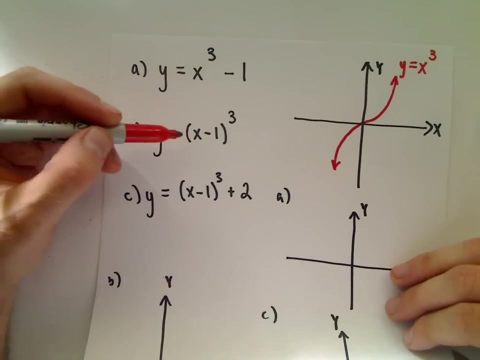 Okay, So kind of a rough little graph there, but hopefully it's making some sense. Let me try to do a couple others here before we run out of time. Same idea Again. So in this case we've got x cubed minus 1, x minus 1 cubed. 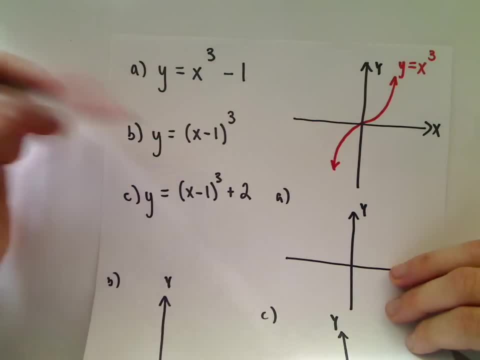 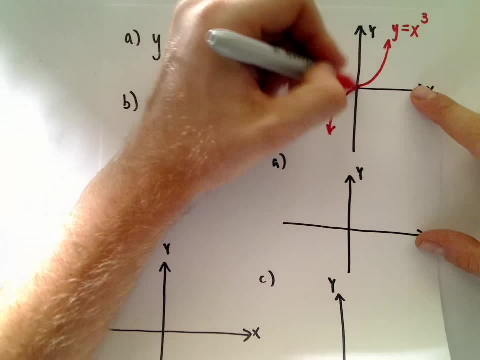 and then x minus 1, cubed plus 2. Again, y equals x, cubed, kind of. our starting point is the graph up here in the top right. It goes through the point Again, part a: x cubed minus 1, all that's going to do to the graph. 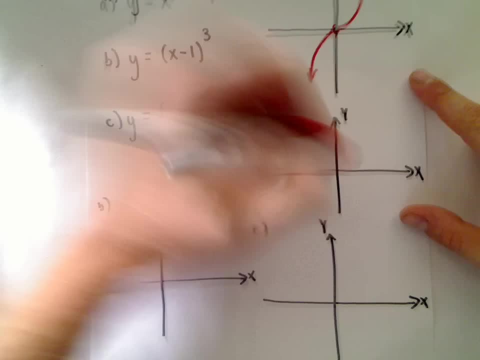 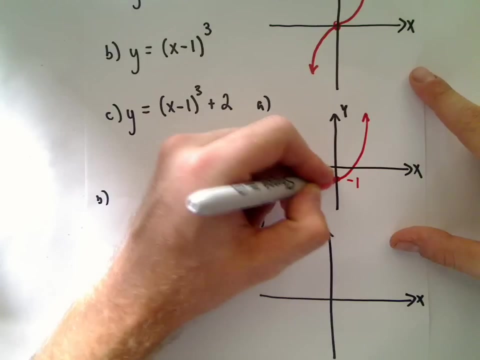 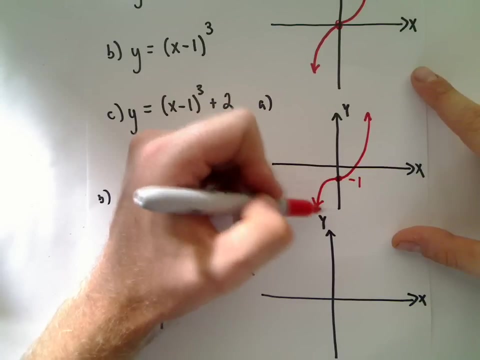 is just move it down 1 unit. So instead of going through, it'll go through And then otherwise it should have that same basic shape to it. Okay, It looks a little flattened out here, So again, I apologize about that. 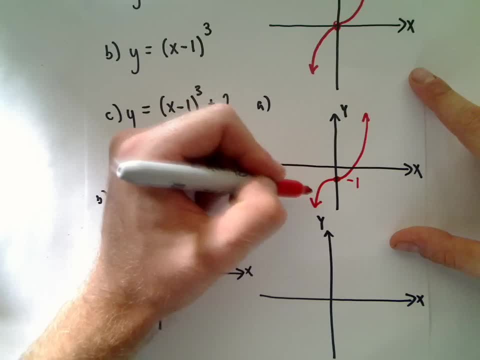 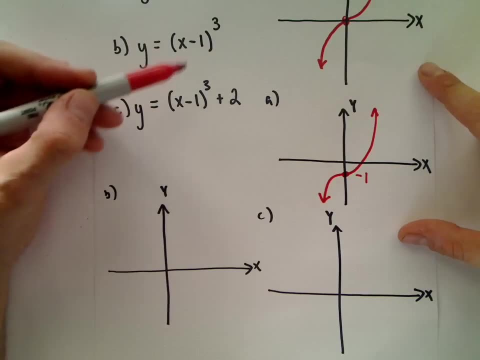 It should be this exact original graph, just moved down 1 unit, So tried to squeeze it in there a little bit and it looks kind of weird. So, part b: the x minus 1 cubed. Okay. So now I replace the x with a negative 1.. 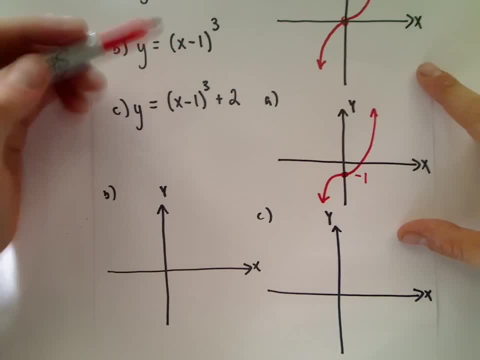 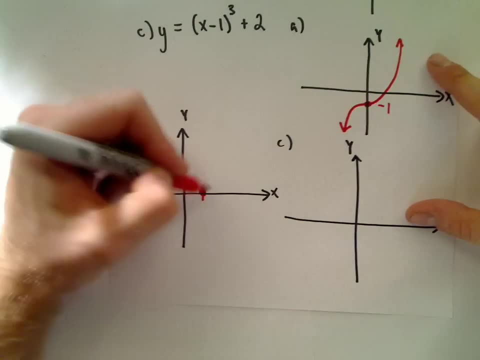 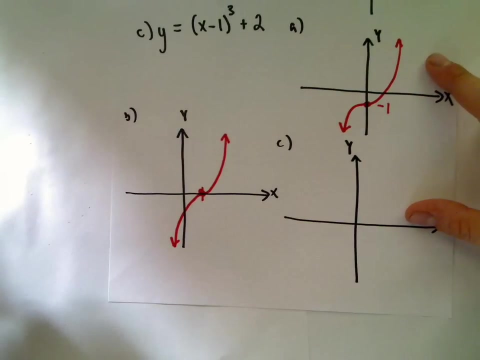 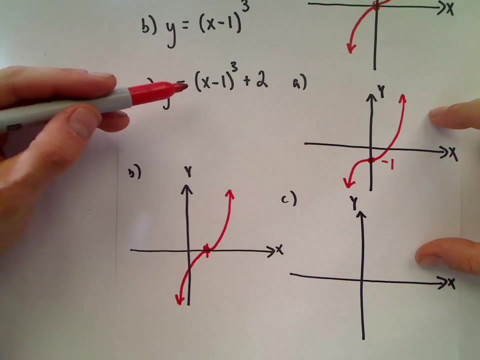 So this is a horizontal shift and it shifts it positive 1 unit to the right. So now, instead of going through, it'll go through And again, still it'll have that same basic shape as x cubed. Last but not least, if we graph x minus 1 cubed plus 2.. 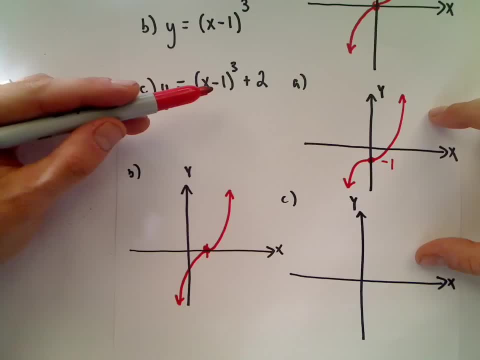 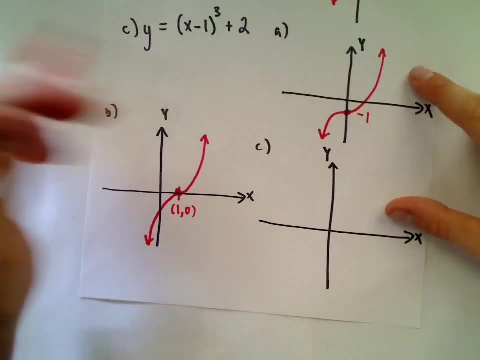 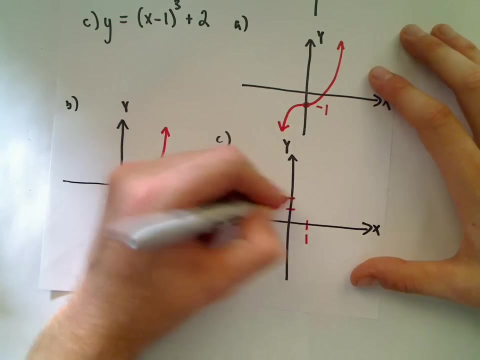 Okay, So all this does is the minus 1 shifts it to the right 1 unit, The plus 2 shifts it up 2 units. Okay, So I can basically just take my part b graph and move that up 2 units. 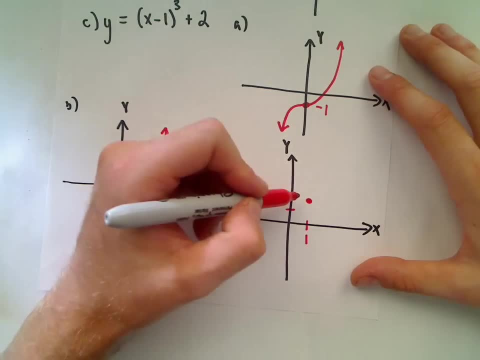 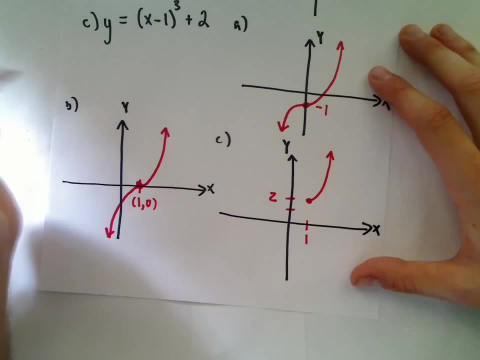 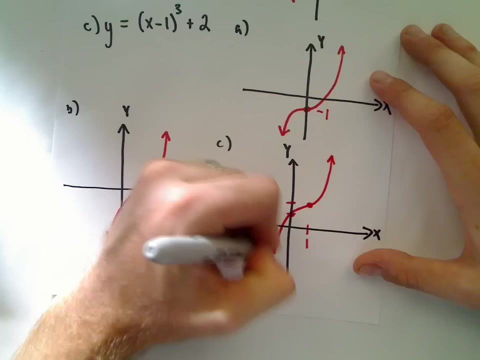 So this point that was originally here at is now going to get moved up to the point. after I move it to the right, 1 and up, 2.. And then again it still has the same basic shape to it. So All right. 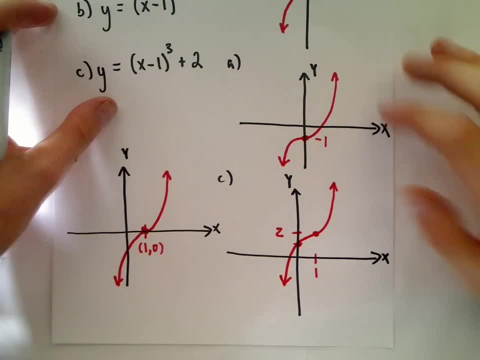 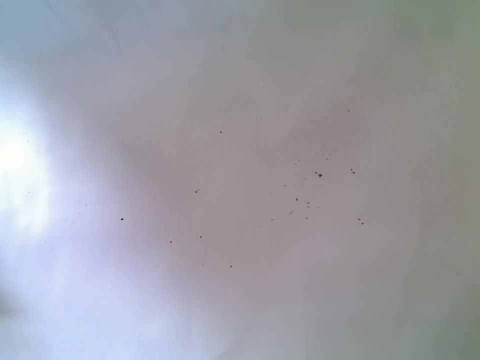 So I hope this makes a little bit of sense here. So it's just recognizing again. have you replaced the x with something or have you just kind of tacked a number onto the outside? So maybe one more little question here. 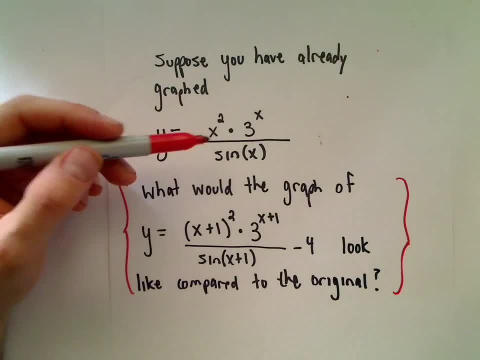 So suppose you already have the graph of x cubed times 3 to the x over sine x. So I'm sure a lot of you looking at this are you know in algebra And maybe you've never seen this function sine of x. 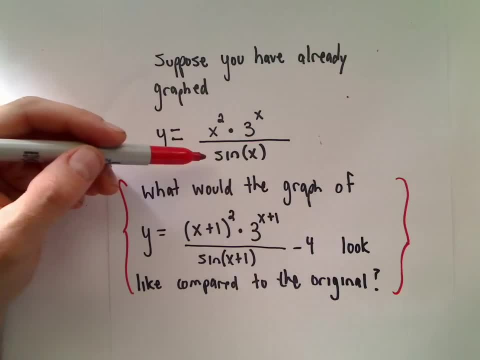 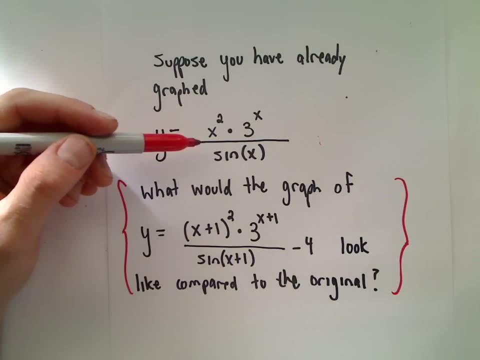 And this is just a trigonometric function, So if you haven't seen it, don't, you know, get too nervous to yet. The main idea again is just: we're replacing x's with what. Okay, So notice. 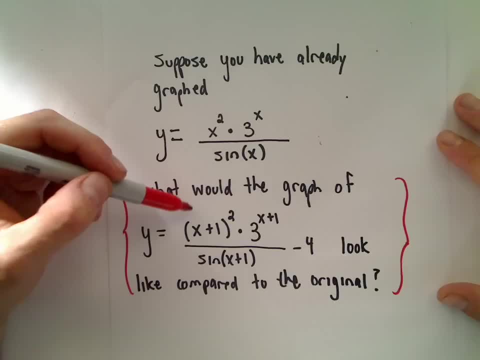 Okay, So I guess I should ask the follow-up. We want to graph now this new graph, x plus 1 squared times 3 to the x plus 1 times sine of x plus 1 minus 4.. We just want to think what would that look like in terms of transformations compared to the original?